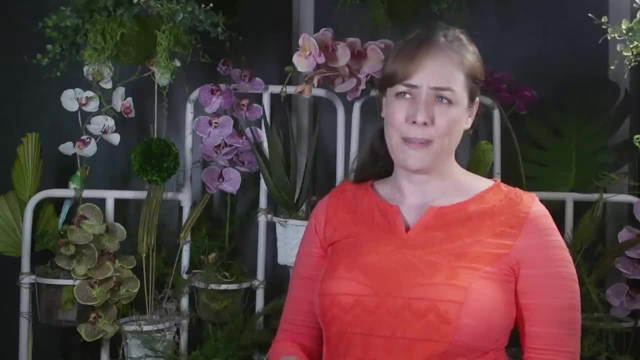 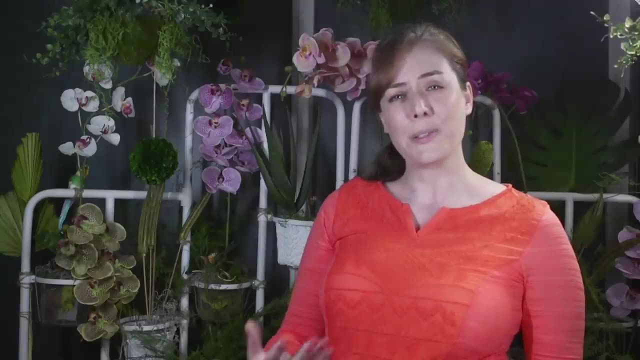 makes sense when the two atoms are identical, Like a hydrogen and a hydrogen share an electron and become an H2 molecule. Or let's look at two oxygen atoms. Neither one has a complete valence shell of electrons. The two hydrogen atoms are the same atom. The two oxygen atoms are the same electron. 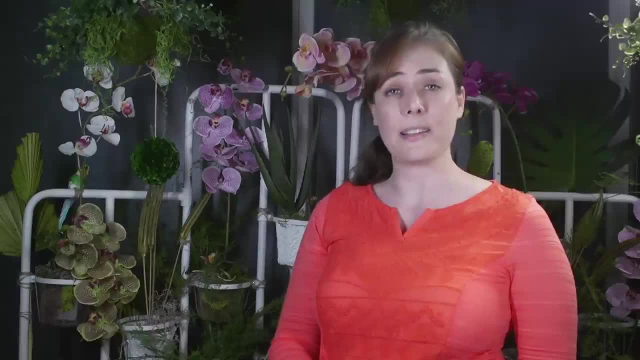 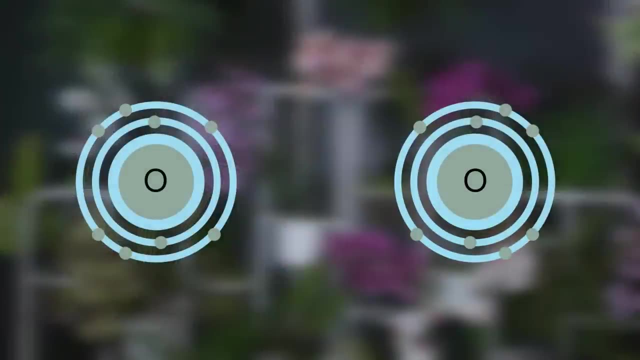 the same electron. The two hydrogen atoms are the same electron and so are the two electronegatives. The outermost valence shell in oxygen has six electrons, so it needs two electrons to fill up that valence shell and become more stable. 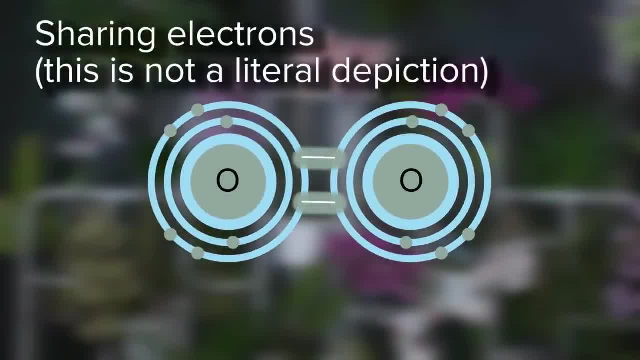 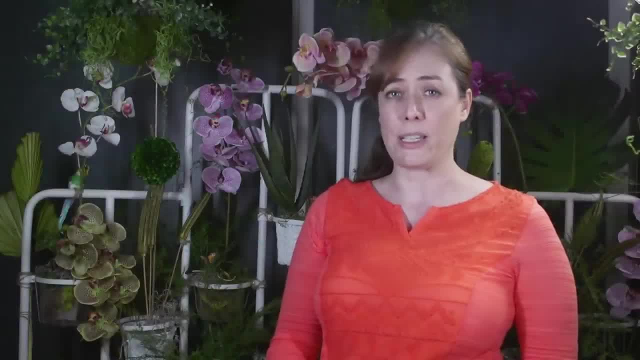 When two oxygen atoms come into close proximity, they can share two electrons and so form a double bond, becoming an O2 molecule. They have the same electronegativity since they're identical, so the electrons are equally shared between the atoms. 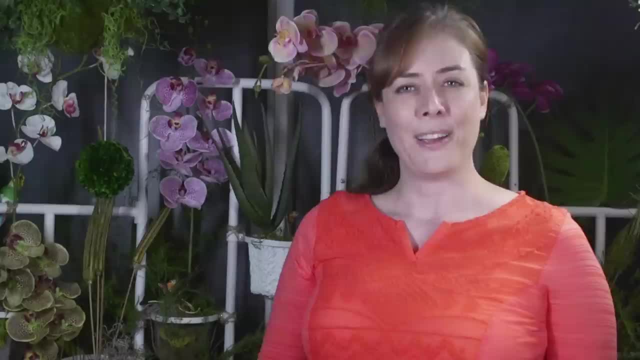 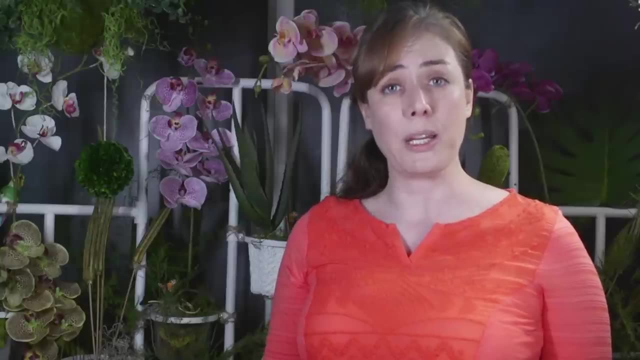 We call this a non-polar covalent bond. Now, if there is a difference in the electronegativities in the two atoms, the electrons will spend a greater amount of time next to the atom with a higher electronegativity. 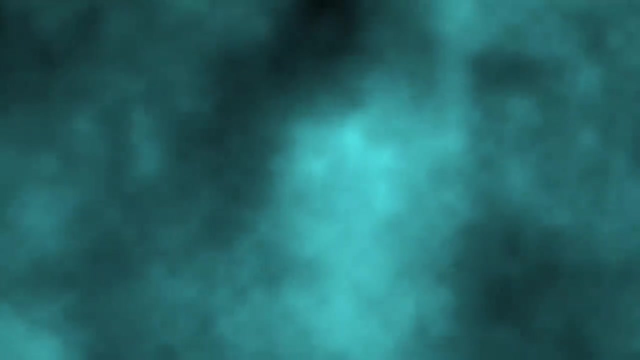 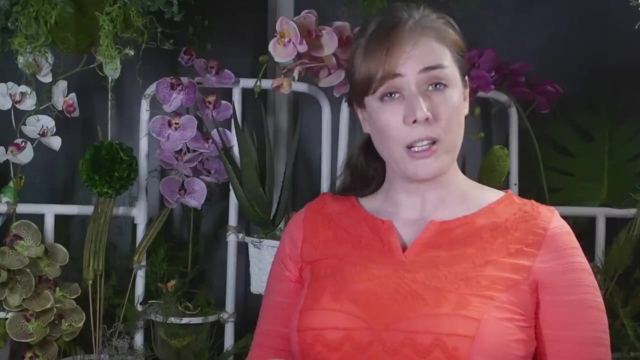 Remember, electrons are always in motion, moving around in kind of cloud-like regions called orbitals. For instance, in a water molecule, H2O, oxygen has a higher electronegativity than hydrogen, So in both of the bonds in this molecule. 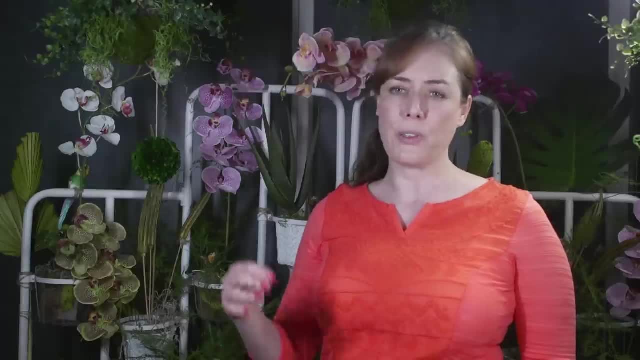 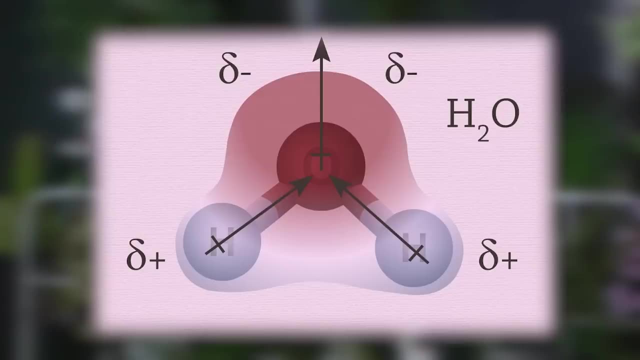 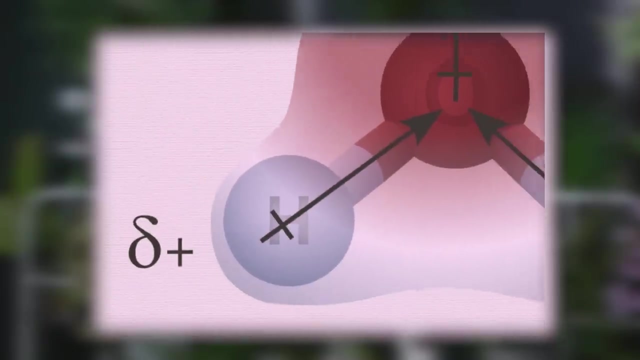 the electrons will spend a greater part of their time closer to the oxygen atom versus next to the hydrogen atoms. This results in a water molecule having a partial negative charge around the oxygen atom and a partial positive charge around the hydrogen atoms. We call this kind of chemical interaction a polar covalent bond. 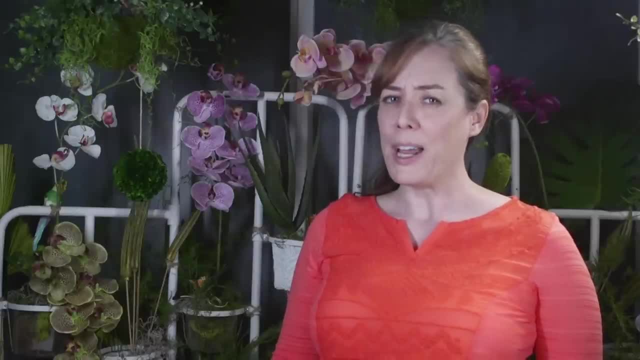 Now, if the electronegativities are different enough, one atom will actually donate one or more electrons to the molecule. This is called an anion: The atom that donates one or more electrons to the more electronegative atom. 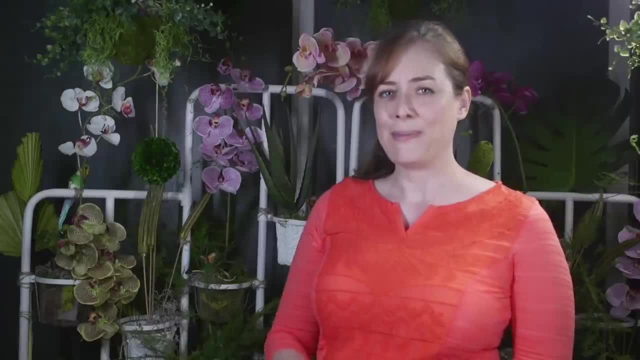 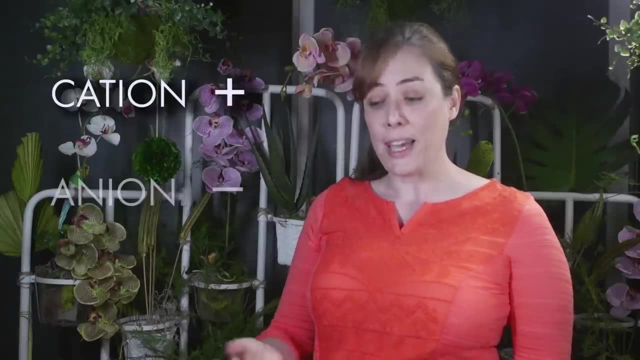 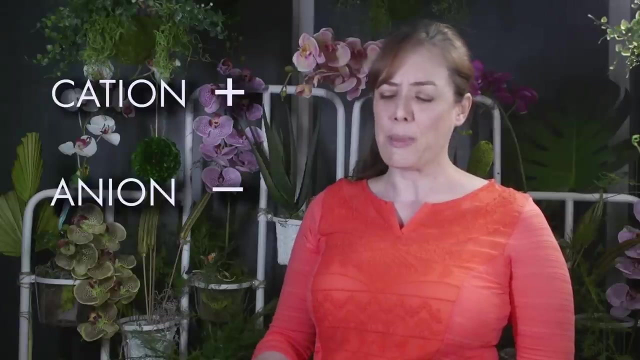 This results in two charged species ions. The atom that donates one or more electrons is called a cation. It becomes positively charged. The atom that takes on electrons becomes negatively charged. This is called an anion. As a result of becoming oppositely charged, these ions are now attracted to each other. 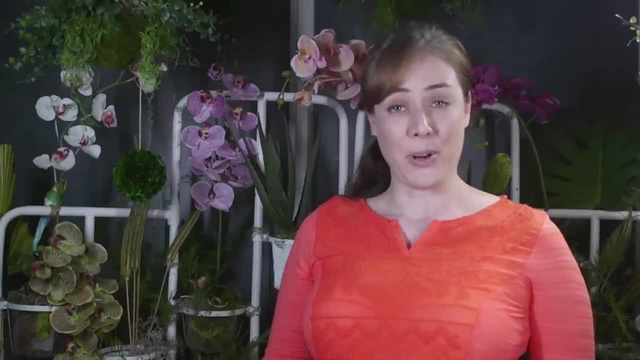 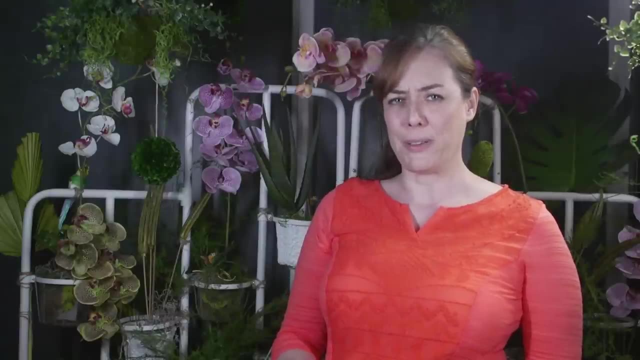 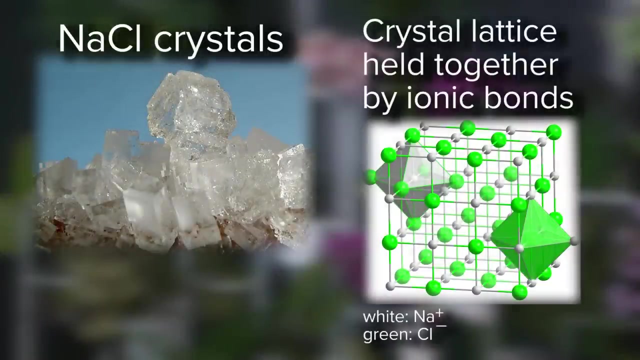 through electrostatic attraction. That attraction holding the two ions together is called anion. Now here's a funny thing about ionic bonds in biology. When you learn about ionic bonds in chemistry, like, say, the bonds holding the salt NaCl together, 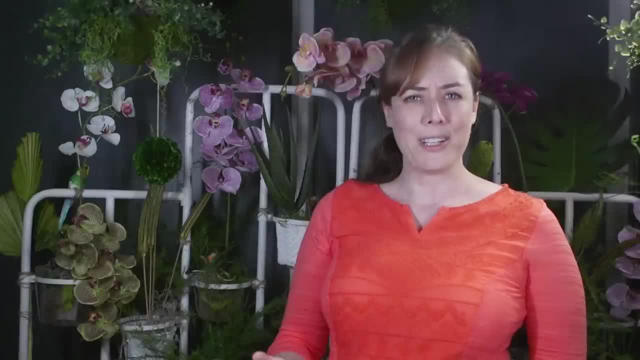 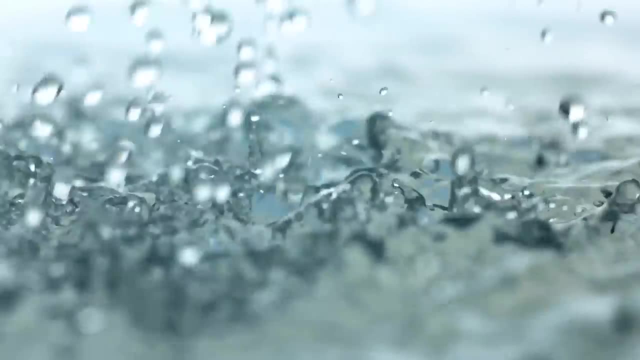 we think of it as quite a strong bond. But in biology, biochemistry, you must remember that everything, all these chemical interactions are taking place in the context of water. In water, ionic bonds quickly dissociate. So for this reason, in biochemistry, ionic bonds quickly dissociate. 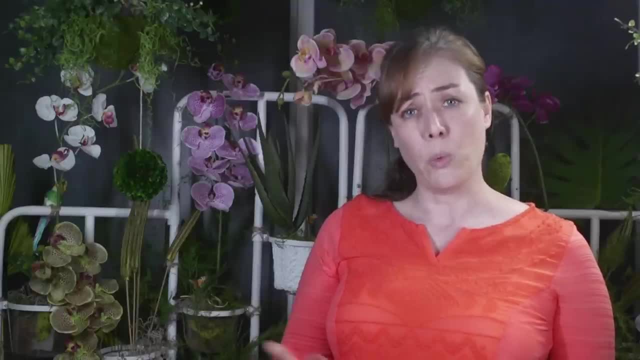 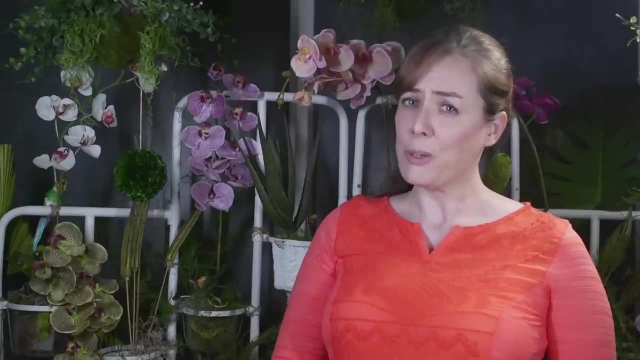 So for this reason in biochemistry ionic bonds quickly dissociate. In chemistry we consider ionic bonds weaker than most covalent bonds. In chemistry we always discuss the range of strengths of these bonds. You can learn more in a video we have called Ionic Bonds versus Covalent Bonds in our 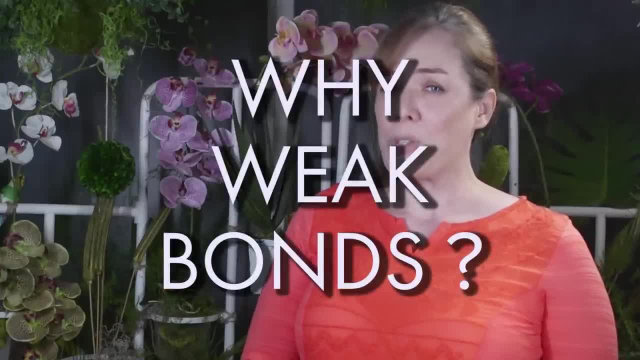 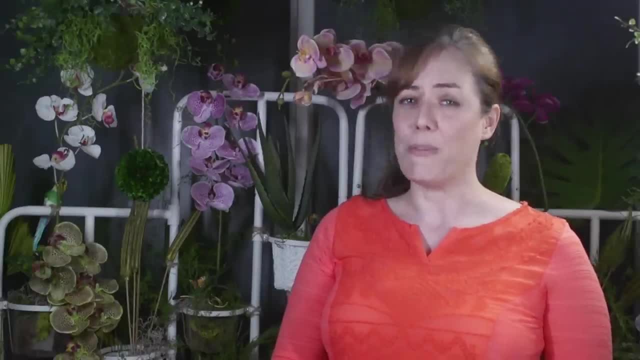 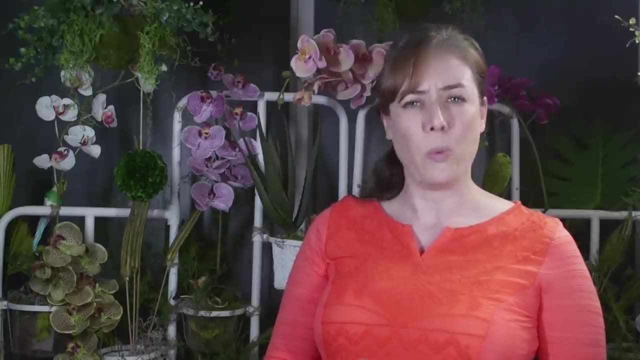 chemistry video series. This may surprise you, but it's really important that we have the capability to make bonds of varying strengths. There are some cases where we want very strong bonds, say, when we're building structures, it makes more sense to have weak bonds, Bonds that can be used for reversible interactions. 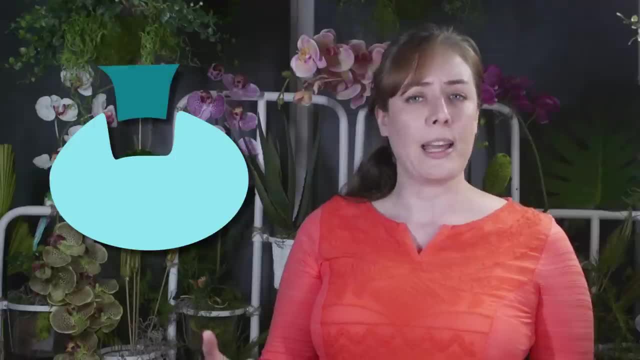 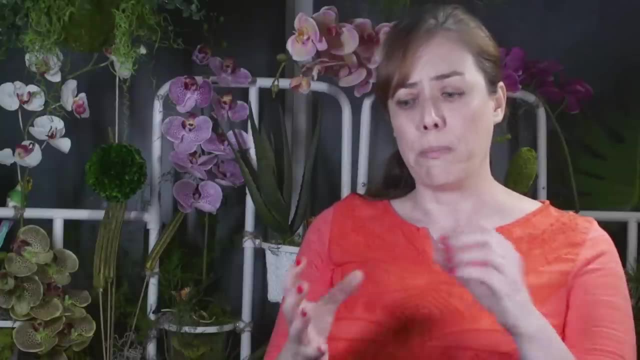 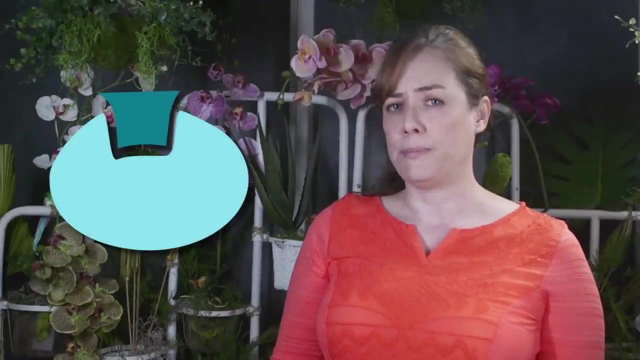 For example, let's say we have a receptor and a signaling molecule that binds it like a hormone or a neurotransmitter. We don't want that signaling molecule to bind to the receptor once and get stuck there blocking the receptor. We want it to bind reversibly. To bind, send the. 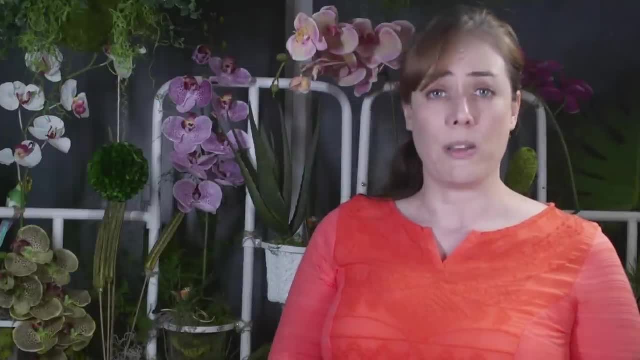 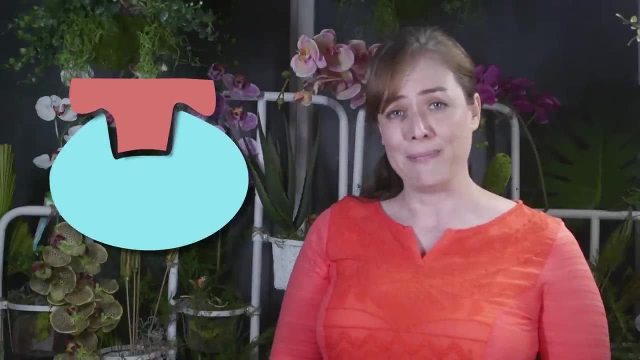 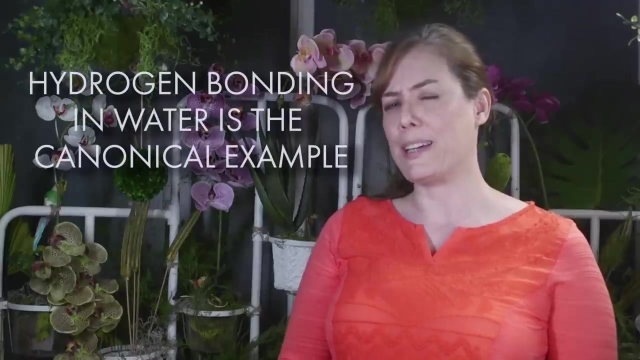 signal and then fall off. In fact, there are some poisons that work this way: They bind permanently to a receptor and they don't fall off, so they mess up signaling in your body. The next weaker bond is the hydrogen bond. People often get confused about hydrogen bonds, because the one 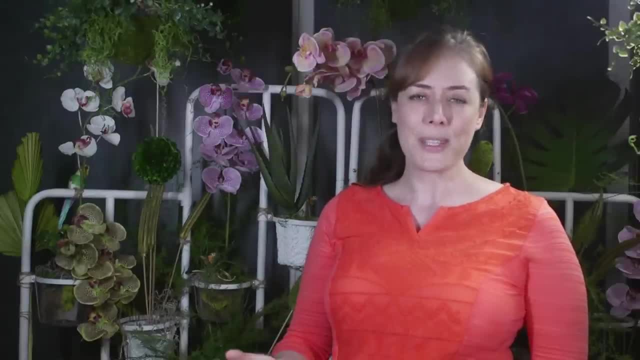 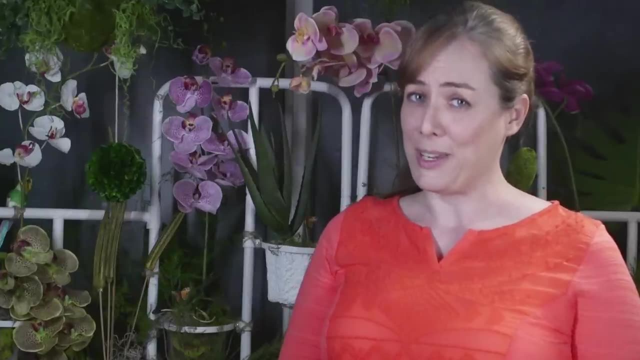 example you'll always hear of is in water. We use that example because it's incredibly important, for why water is essential to life, and that's a topic for another video. But meanwhile the confusion comes because we just said there are polar covalent bonds. 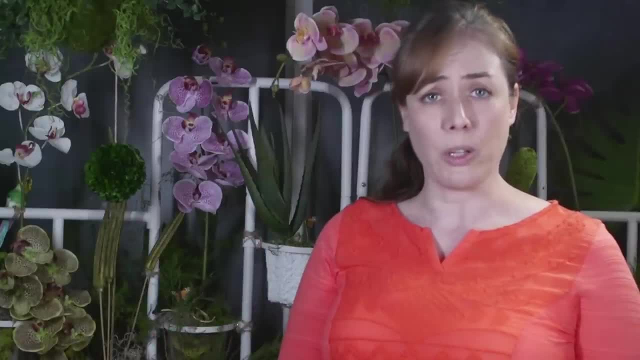 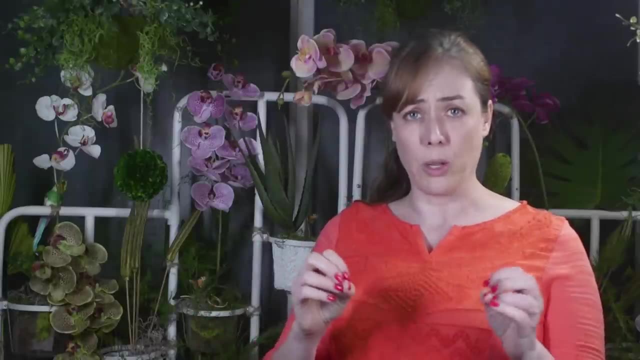 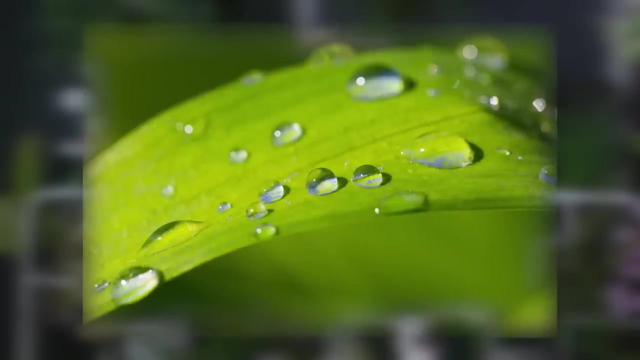 in water. Yes, in individual water molecules. those bonds are polar covalent bonds. There are hydrogen bonds that hold different water molecules together. This is what makes water so cohesive, For example, why water forms drops that kind of bunch up instead of lying flat. 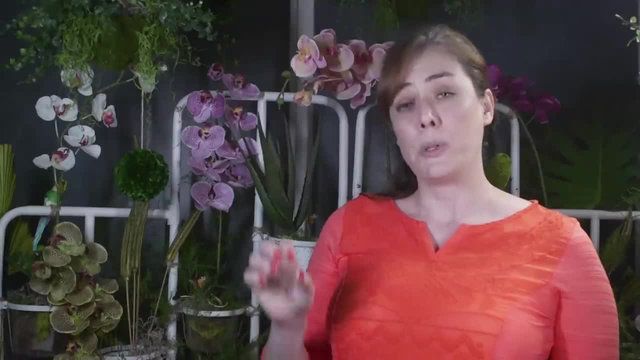 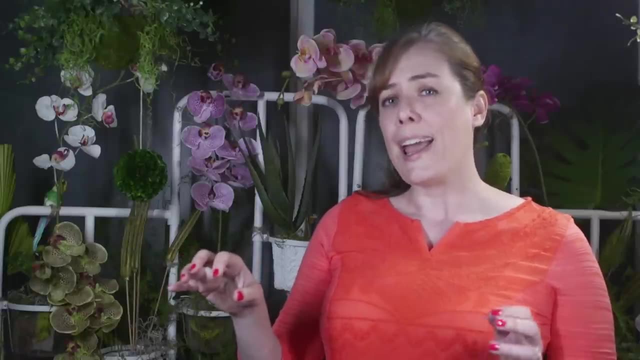 The hydrogen bond is the very weak attraction. Between one and two, the hydrogen bond is the very weak attraction. There's one hydrogen atom that's already covalently bonded to something else, so it has a partial positive charge and something else that is partially negative. This is usually an oxygen. 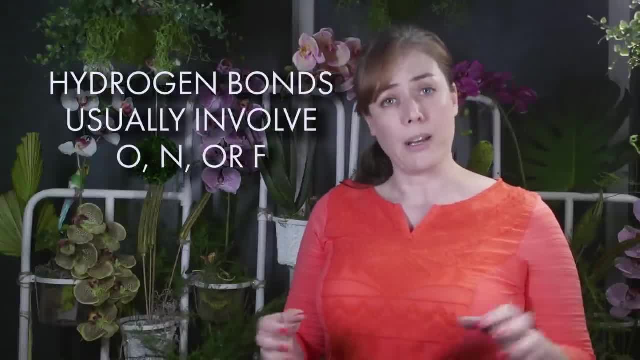 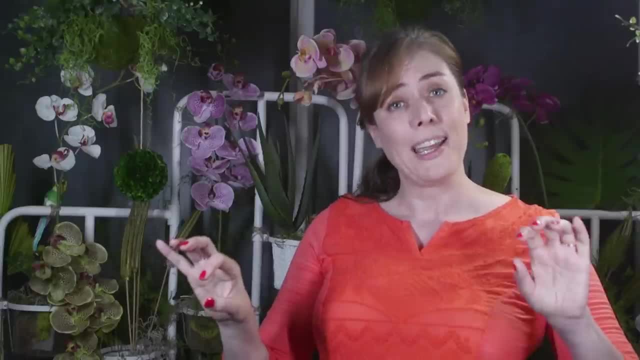 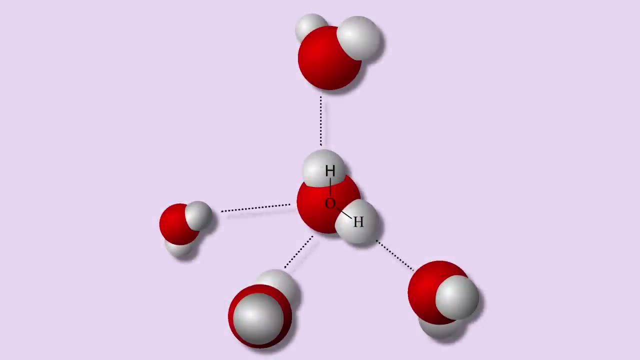 nitrogen or fluorine atom that is bonded to something else. So in the case of water, you have the hydrogen from one water molecule attracted to the oxygen in a different water molecule. Notice that these bonds are written differently from covalent bonds. Rather than a solid line, 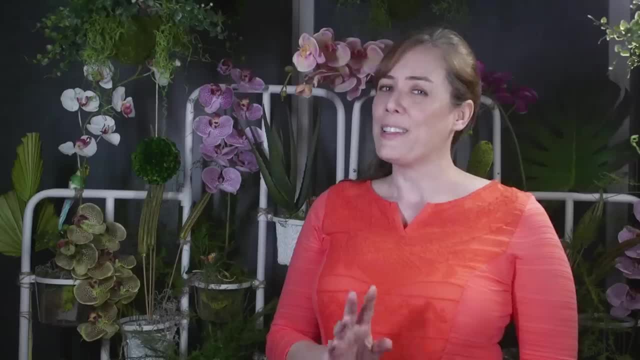 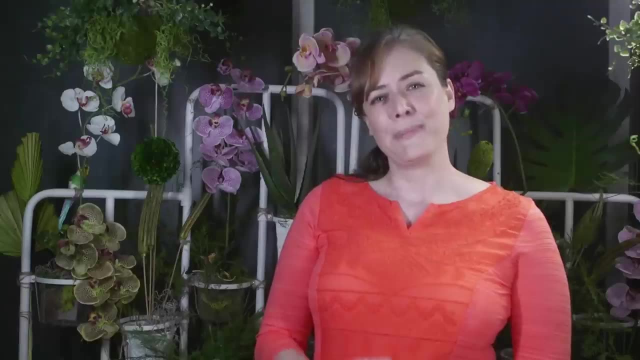 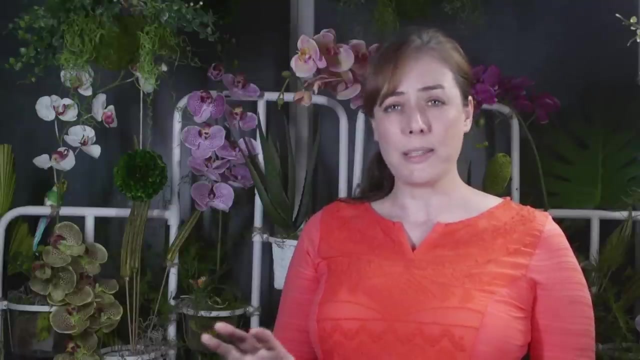 joining the two atoms. it's a dotted line. That's to remind you that this is a very weak interaction. These bonds kind of blink on and off. Now let's talk about the very weakest kind of bond, the van der Waals interaction. To understand these, you must keep in mind the idea that electrons are 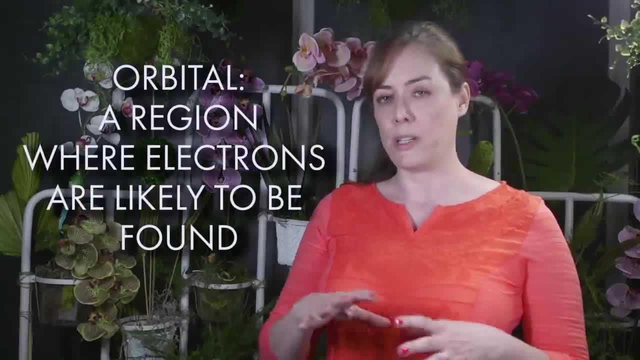 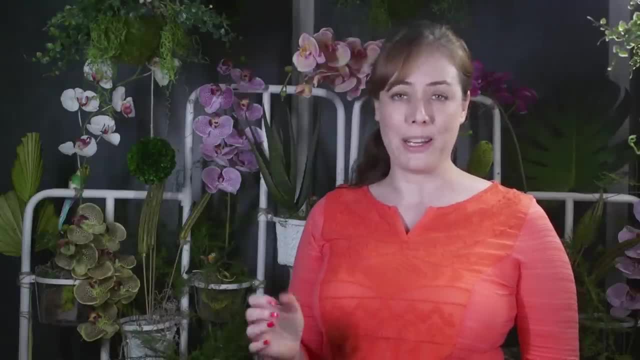 constantly in motion. They occupy an orbital which is a cloud or a region around their atom's nucleus. You can't pinpoint exactly where they're located, but you can see that they're in motion. You can't know exactly where it's going to be at any one moment, but you have an idea of this region. 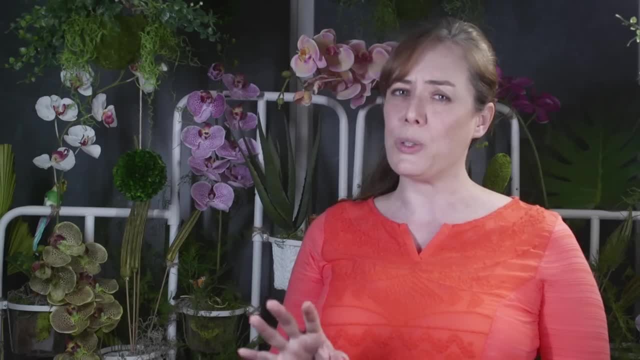 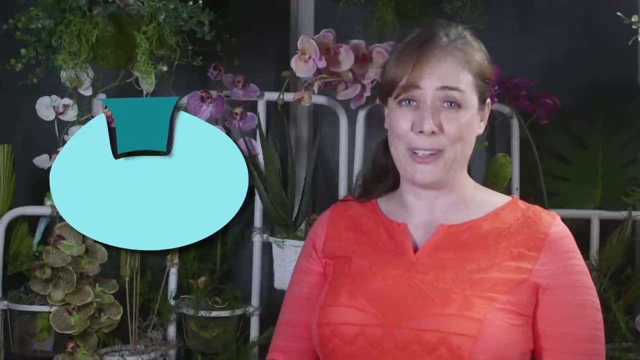 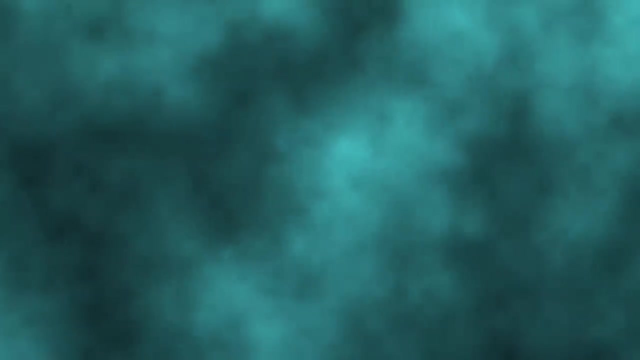 where you can find it with high probability. So now imagine two typically bulky molecules coming into contact, or that receptor and signaling molecule that we mentioned earlier. On the surface, the very, very surface, there's a cloud of electrons moving around Some of the time. 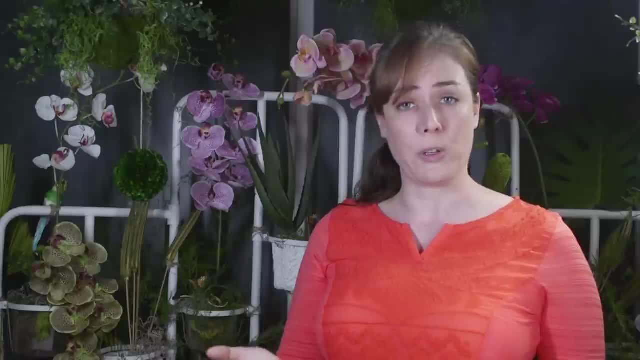 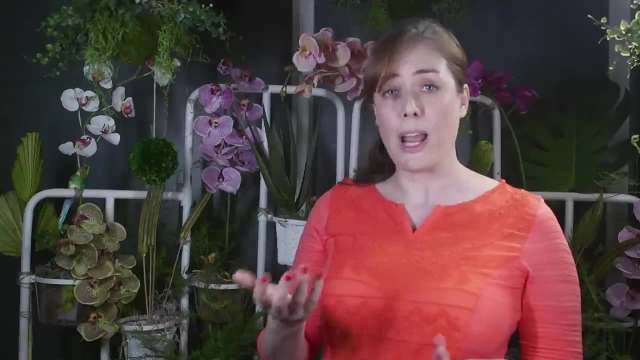 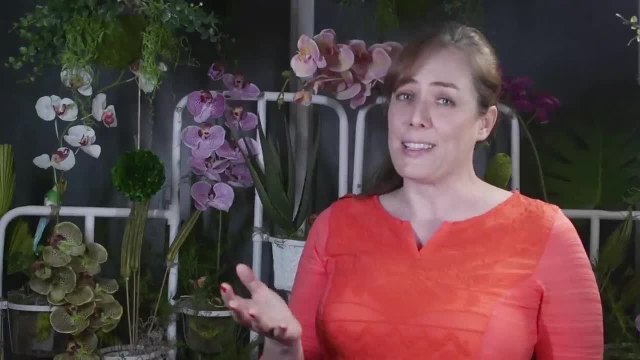 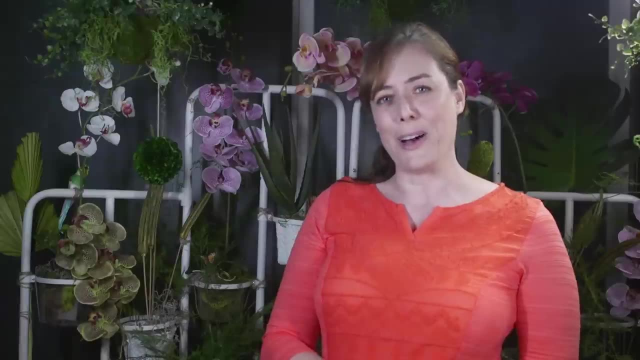 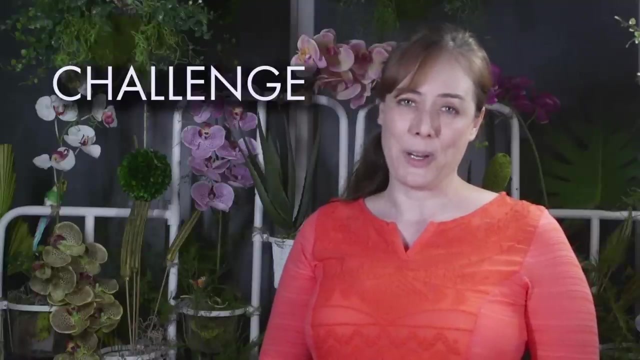 and briefly be attracted to each other, And then in the next instant they're released Again, sort of like the hydrogen bonds. Imagine these bonds twinkling on and off like Christmas lights, except now even faster. Here's a challenge for you, For each one of these kinds of bonds.